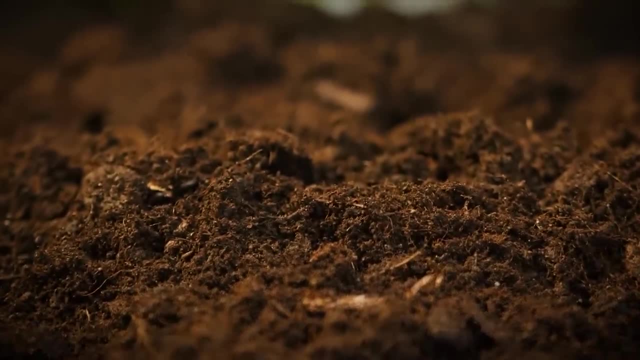 since soil without forest and grass gets washed out and eroded quickly, and it will take hundreds of years for the rabbits to grow back to their natural habitat. This is a terrible thing to do. Years have passed since the rabbits were born, but they are still alive. 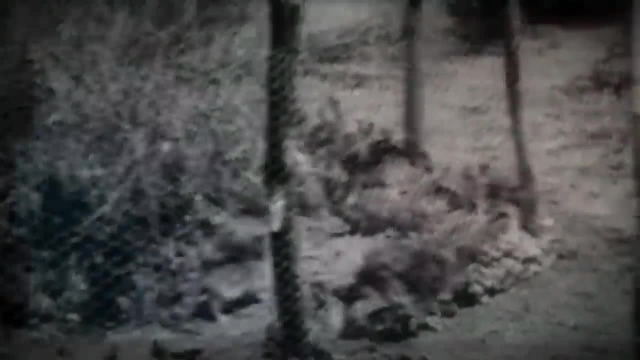 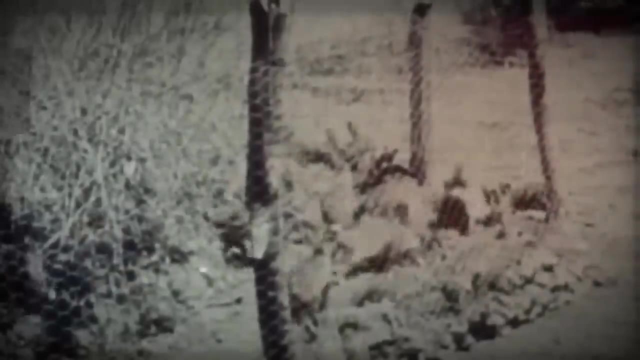 Several methods were used to try to decrease the rabbit population. They were shot, poisoned and their holes were plowed up with tractors, But none of these measures have proven to be effective. In 1950, a biological weapon was used against rabbits for the first time. 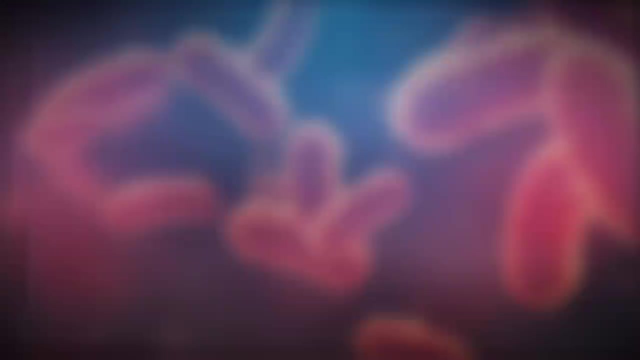 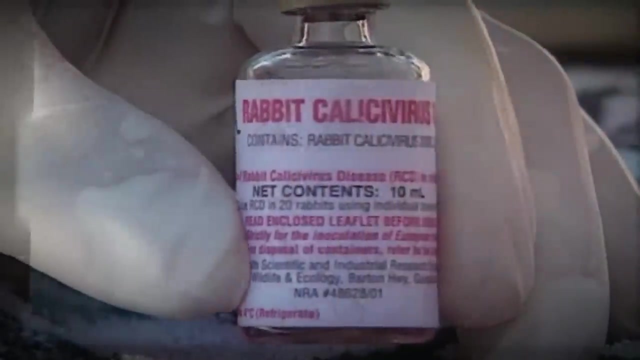 It was the myxoma virus. 99% of the rabbits died from the disease at the time, but the survivors developed resistance to the virus. In 1995, a biological weapon was used against rabbits for the first time. This was the calyxivirus, which causes rabbit hemorrhagic. 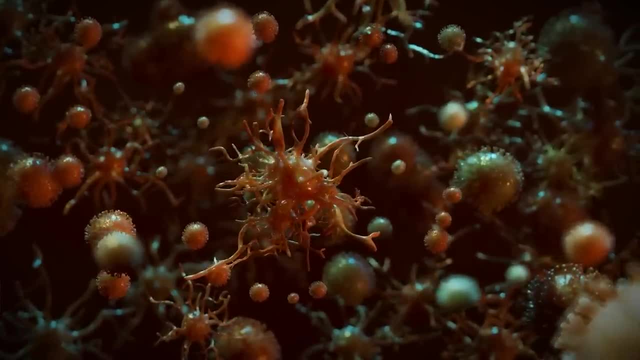 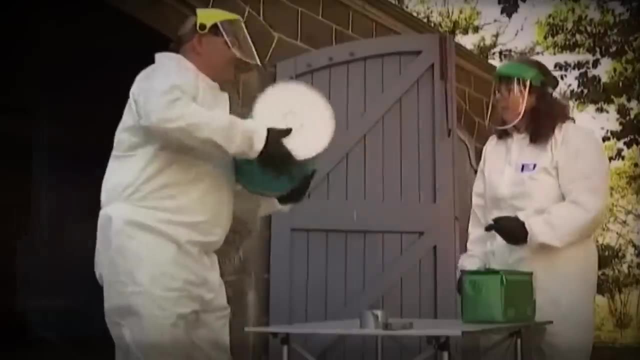 disease. This virus helps keep the wild rabbit population within the 300 million mark. A few years ago, another virus was released to fight Australian rabbits. It's a Korean stamp that Australians hope will help them further reduce the number of rabbits on the continent. 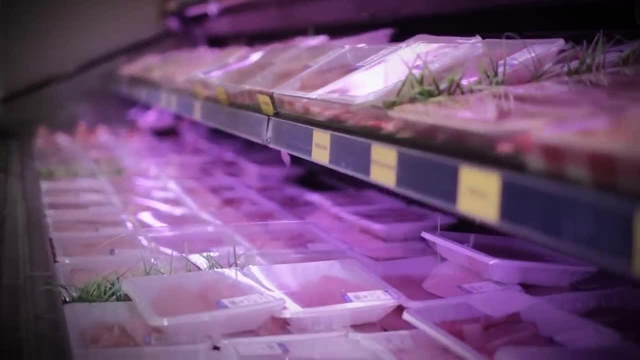 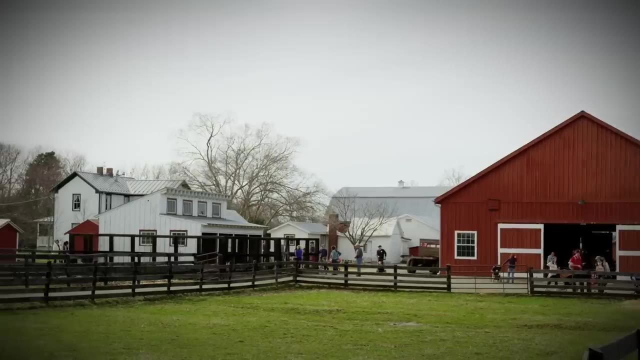 So how come there are so many rabbits in Australia but their meat isn't sold in stores? It turns out that only a few thousand rabbits were kept in private households. There are only four farms in all of Australia where they are bred. The problem is that all of the released 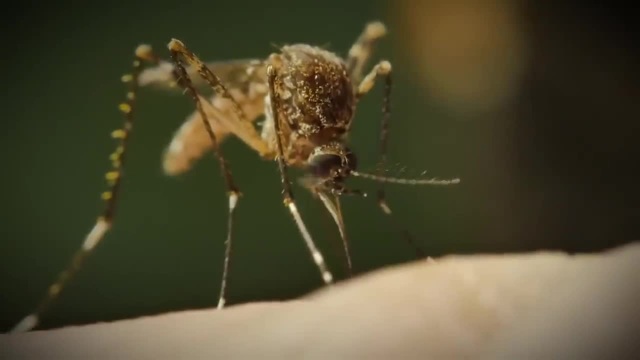 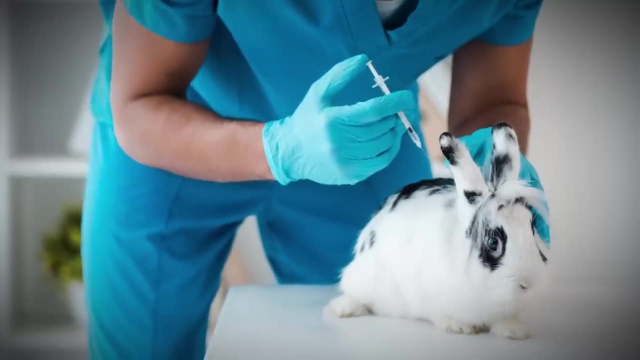 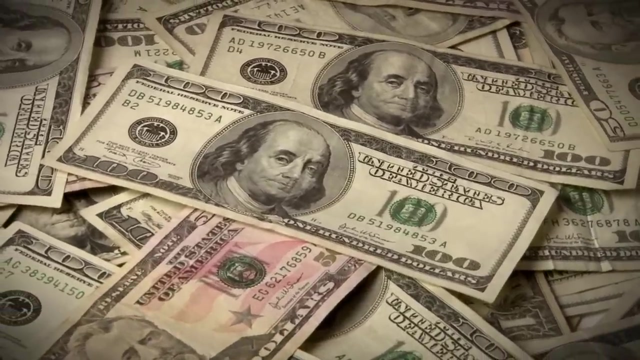 viruses are carried by blood-sucking insects that don't distinguish between wild and domestic rabbits, but simply infect all of them. It costs $10 to vaccinate one rabbit and $40 if the vaccination is done by a vet. Thus, the breeders would need to spend $10,000 to $40,000 a year. to vaccinate a farm of 1,000 rabbits. That's just too expensive. Therefore, rabbit meat in Australia is considered one of the most expensive kinds of meat, which are only served in fine dining restaurants. As for the meat of the wild rabbits, first of all, they are all infected. 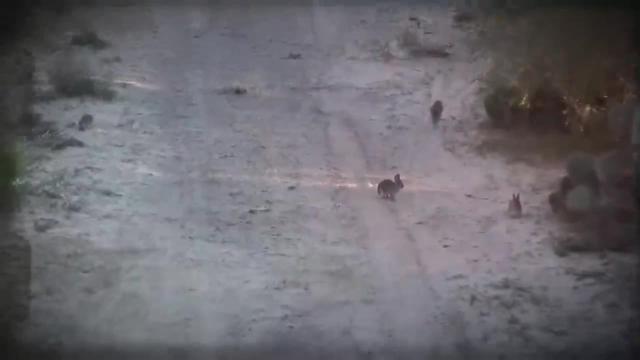 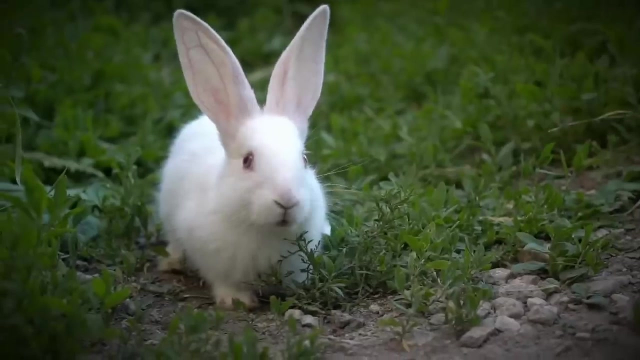 and no one wants to eat the meat of sick animals. And second of all, those rabbits are wild, which makes their meat tough and sinewy, so it has no culinary value. So that's the secret: Australians treat rabbits the way we treat rats and we don't eat rats.